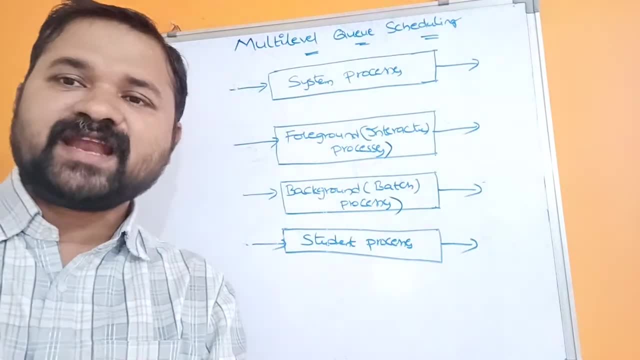 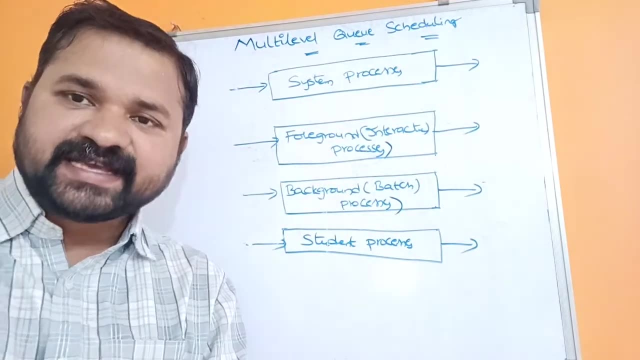 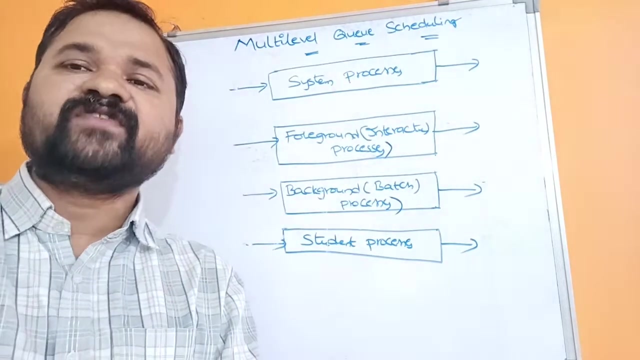 In this video, we are going to discuss about multi-level queue scheduling algorithm. We have different types of scheduling algorithms like FCFS, SAF, Round Robin, Priority, SRTF scheduling algorithm. In every scheduling algorithm, we will use as only one ready queue, whereas a multi-level 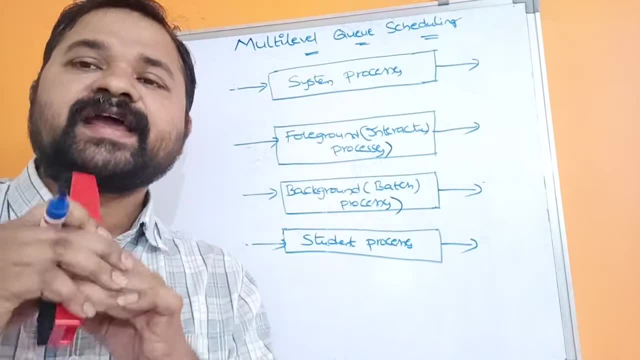 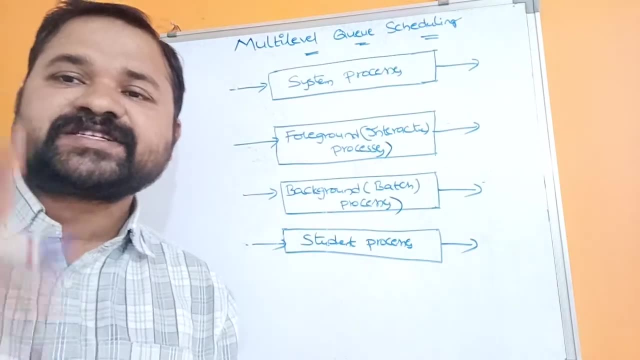 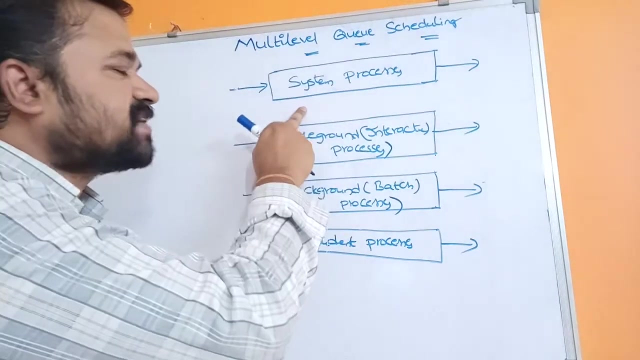 queue scheduling algorithm partitions a ready queue into multiple ready queues, So here we can have multiple ready queues instead of only one ready queue. Let us observe this diagram. Here we have four ready queues. The first ready queue stores system processes. The second ready queue stores. 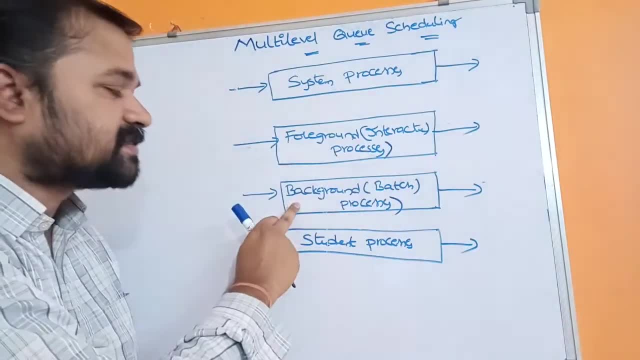 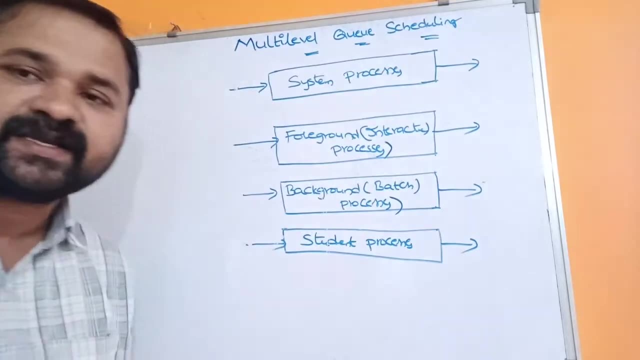 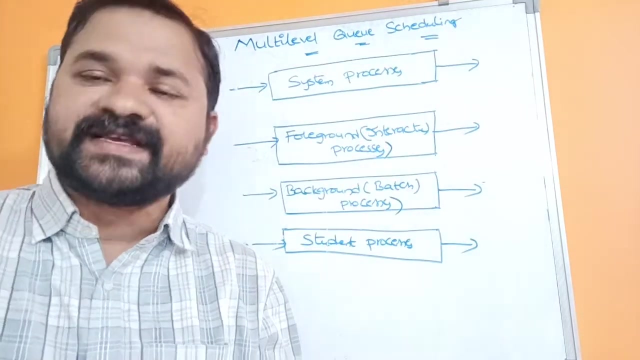 foreground or interactive processes. The third ready queue stores background or batch processes. The fourth ready queue stores system processes. Here a process will be stored in the ready queue based upon the process properties. Here the process properties are size of the process, CPU burst. 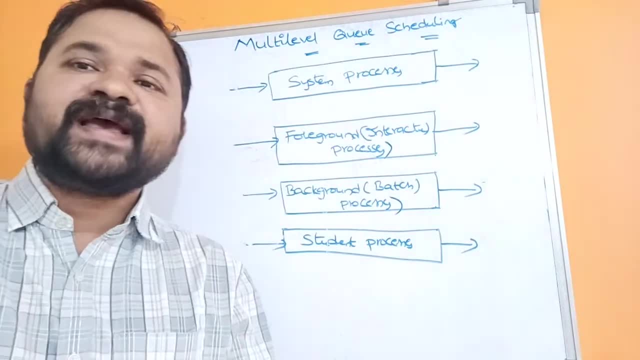 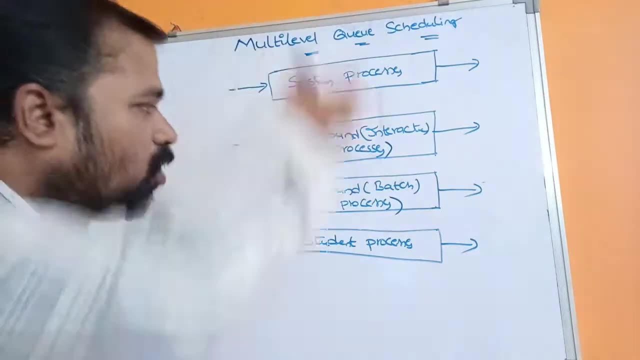 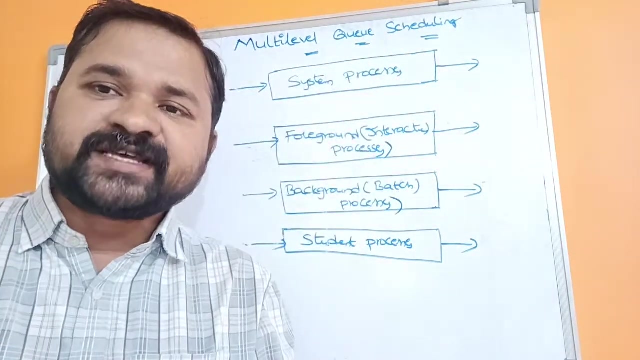 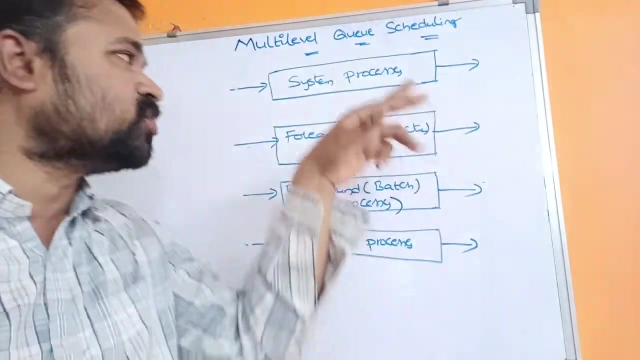 time, priority, etc. So, based upon those properties, the processes will be stored in the ready queue. Let us understand what all these processes are Here. the first ready queue stores system processes. System processes means in order to use operating system, we require some processes. So all those processes will be stored in in this ready queue And the 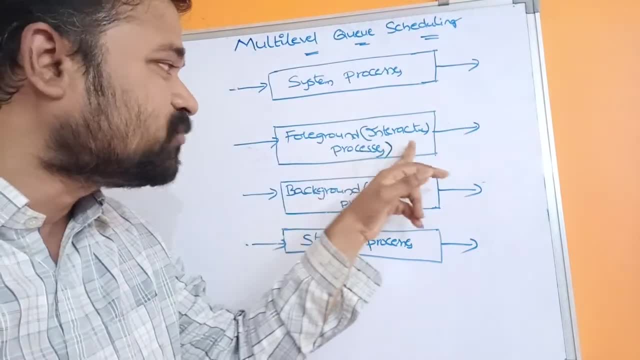 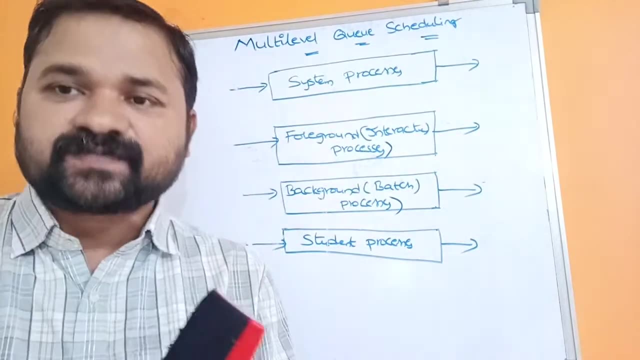 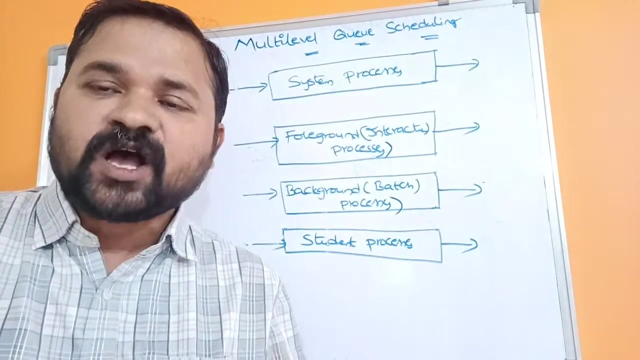 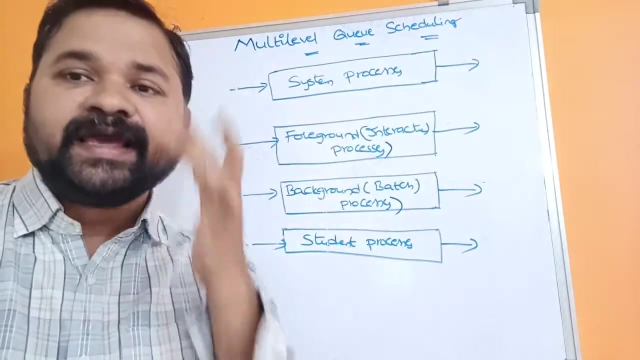 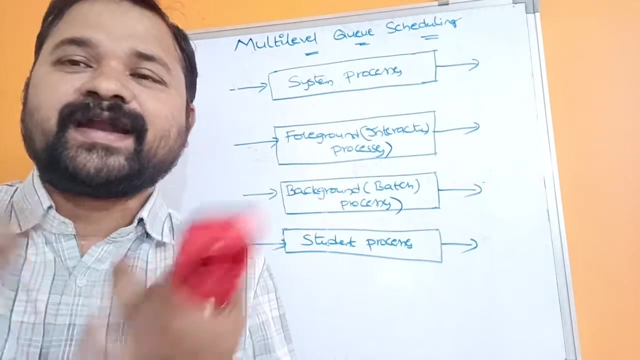 next ready queue, stores, foreground or interactive processes. Interactive process means that process response time is very, very less, So the system has to produce the response in a faster manner. If you take the example of play cards game, if you make any move then the system has to make its move in a faster manner. So any game is nothing but an interactive process. So all those important and interactive processes needs to be placed in this study queue. 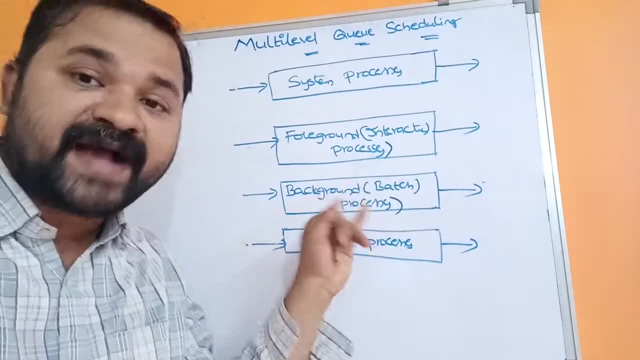 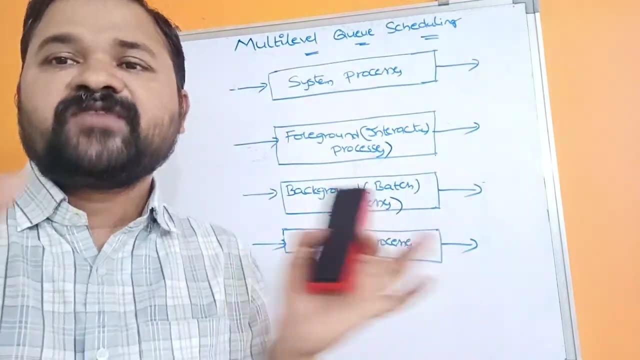 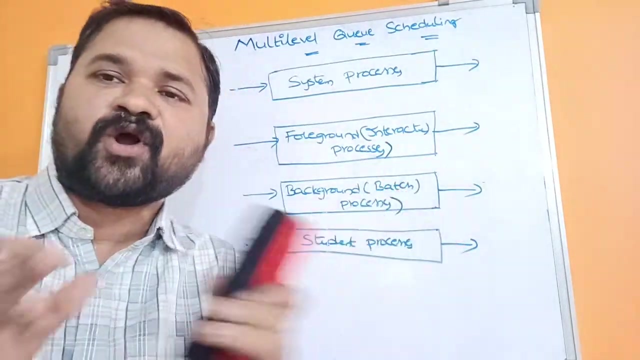 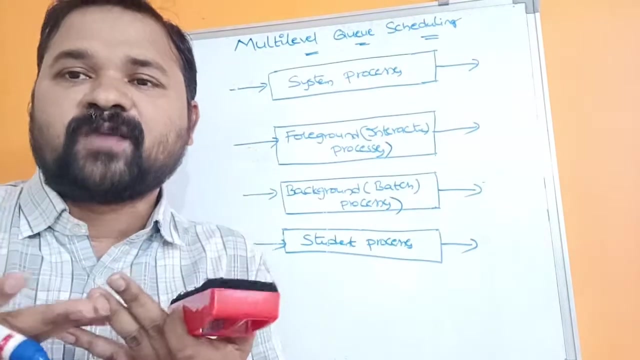 And the study queue stores background or batch processes. So batch process means that process response time is not a matter. If the system produces response for taking long time, then there is no problem. Why? Because these processes are not that much important, And the last one is student processes. So if we develop any program, then that is nothing but a student process. 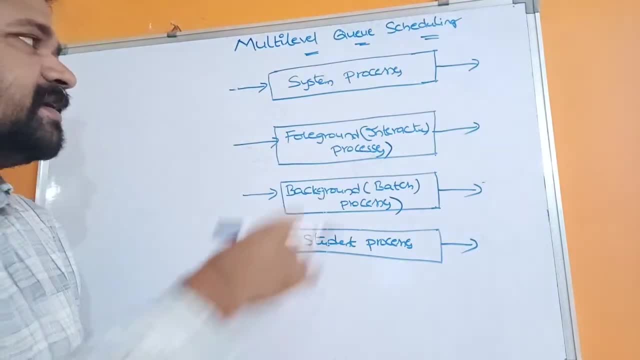 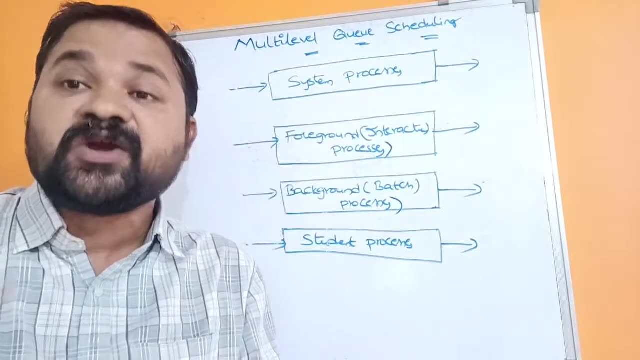 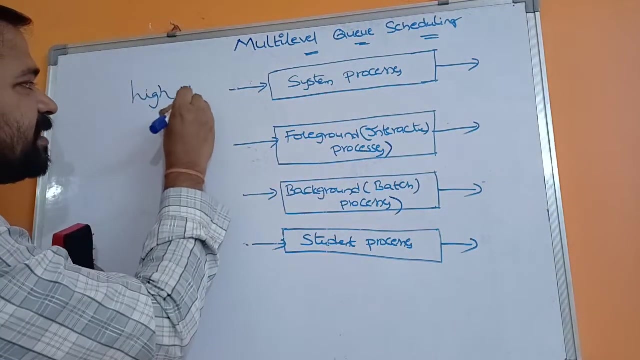 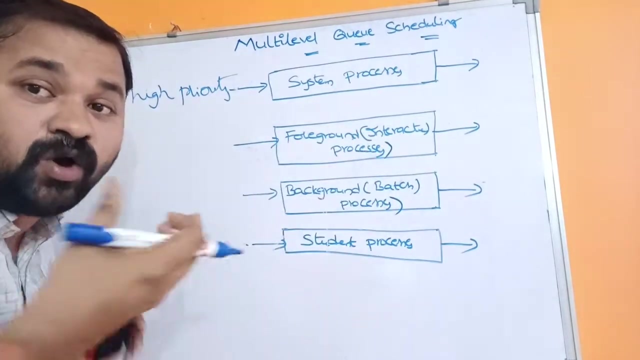 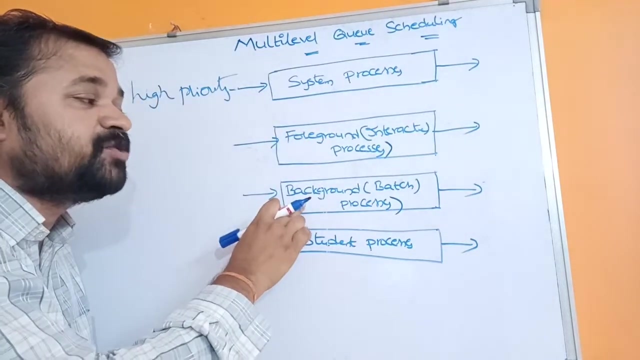 Now here, out of all the all these ready queues, system processes are very, very important. Why? Because we are using these processes in order to run the operating system. So a high priority will be given to the system process. A high priority will be given to the system process Next. next, foreground, interactive processes are very, very important. So, next, high priority will be given to the foreground processes. Next, high priority will be given to the batch processes. 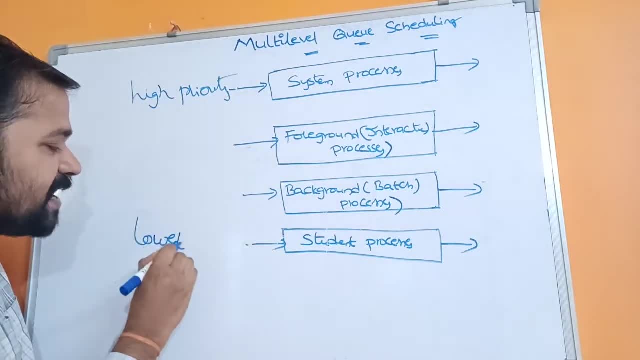 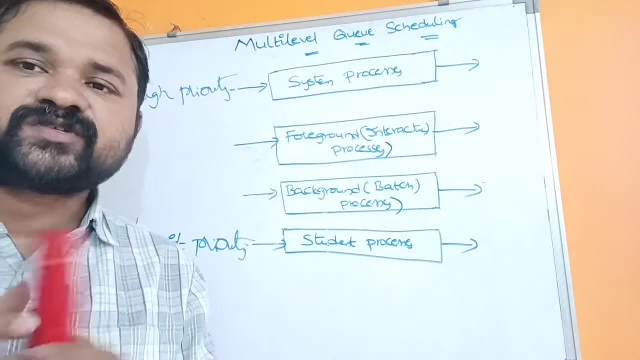 And then, second, the whole of all the video will be given to the system processes Next, next priority will be given to the student process, Where, as the lowest priority will be given to the student processes, Ok, so likewise, the priorities will be given to all the ready queues. 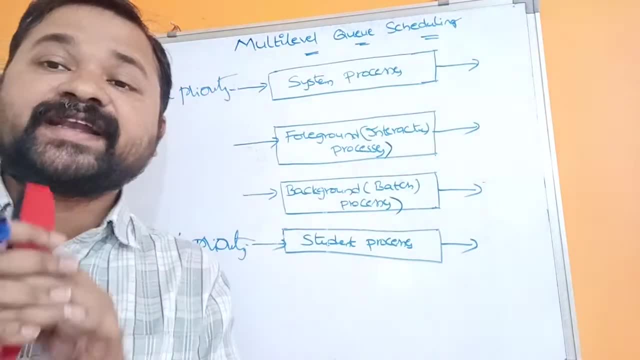 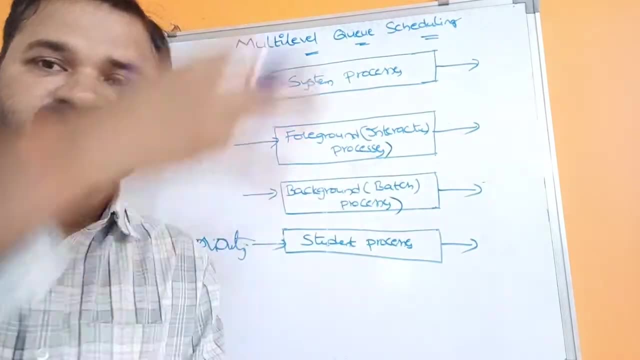 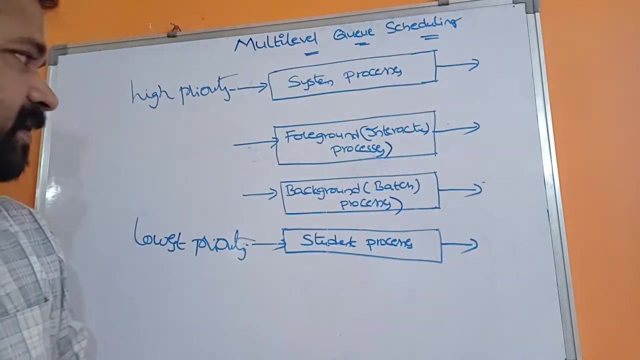 Here each ready queue has its own scheduling algorithm. So our each ready queue we can apply our own scheduling algorithm. So on each ready queue we can apply our own scheduling algorithm. So we have several scheduling algorithms: FCFSSAF, downrobin priority- We can apply our own algorithm here. 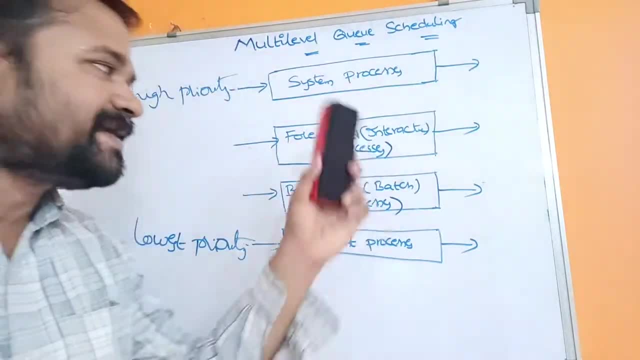 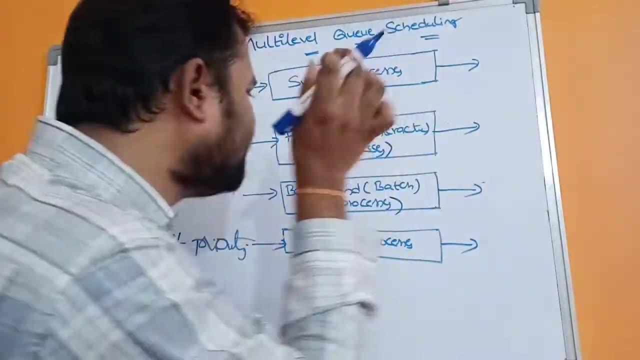 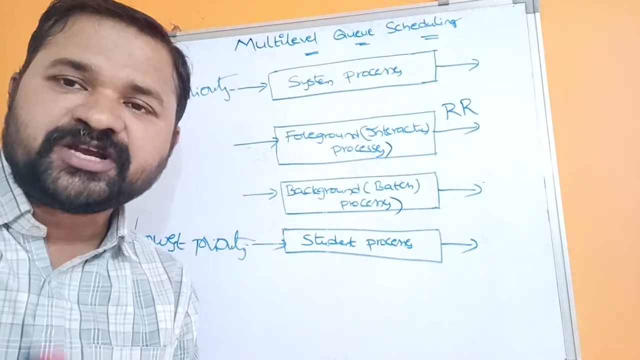 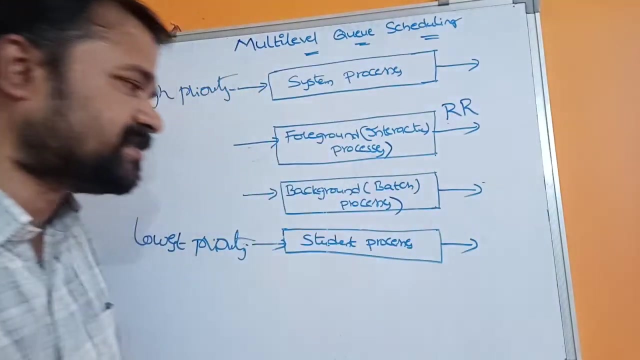 let us observe interactive and batch processes. interactive means the response time should be very, very faster. okay, so here on this ready queue, it is better to apply round robin scheduling algorithm. why? because round robin scheduling algorithm produces the response in a faster manner, whereas, coming to the batch processes, it is better to schedule these processes with the 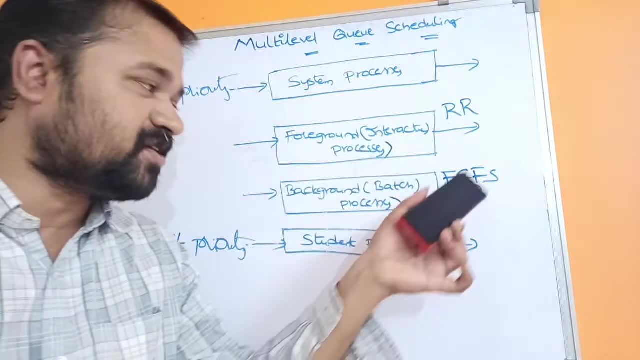 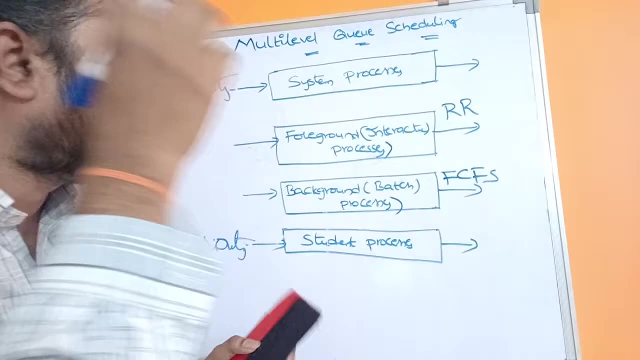 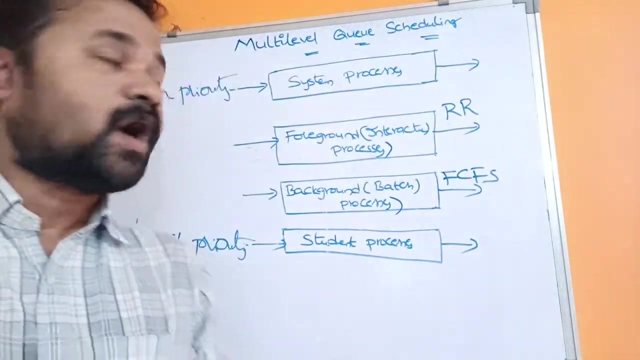 help of fcfs. and either why? because fca. if he uses fcfs, then it produces the response by taking too much of time. so likewise we can schedule the radius with the help of the corresponding algorithms. and one more important point is how we can perform the scheduling between different queues. 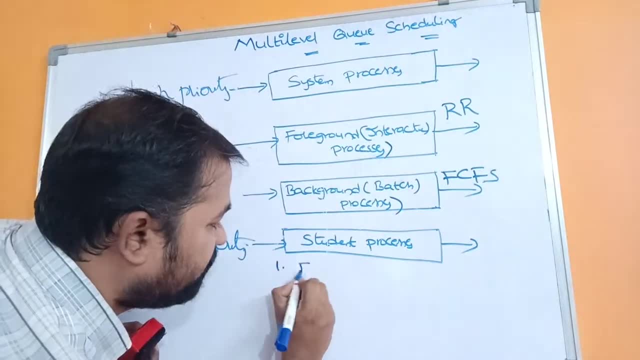 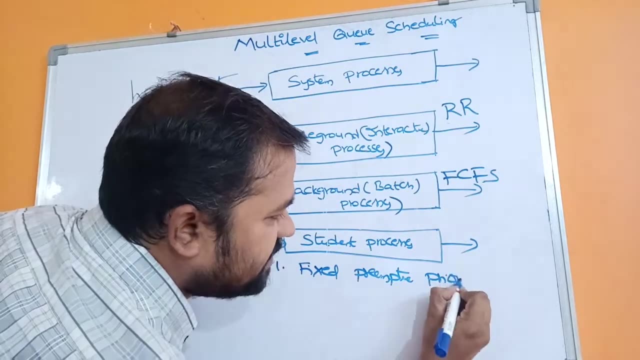 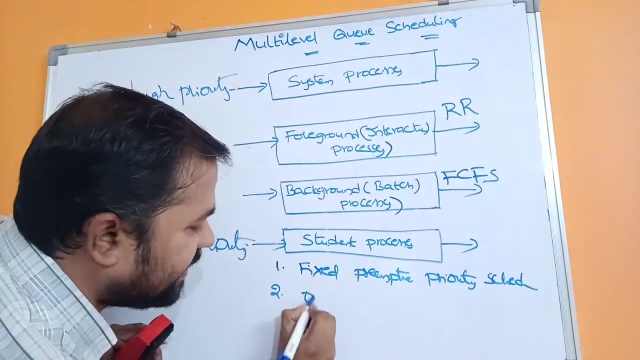 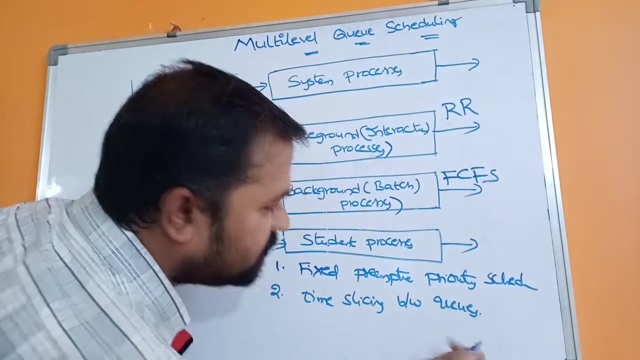 for that, totally. we use two approaches here. the first one is fixed primitive priority scheduling algorithm. so this is nothing but primitive priority scheduling algorithm. and the second one is time slicing- time slicing between the queues. so here the point is how we can schedule between different queues. for that we use just two. 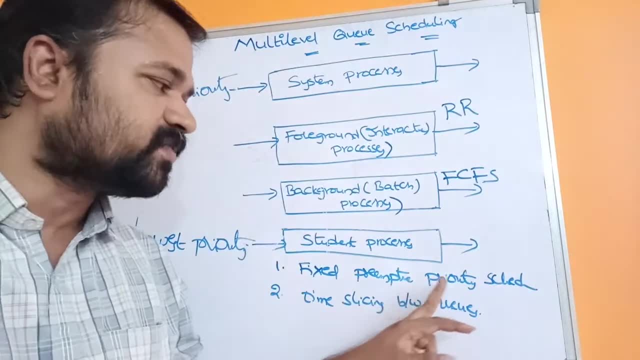 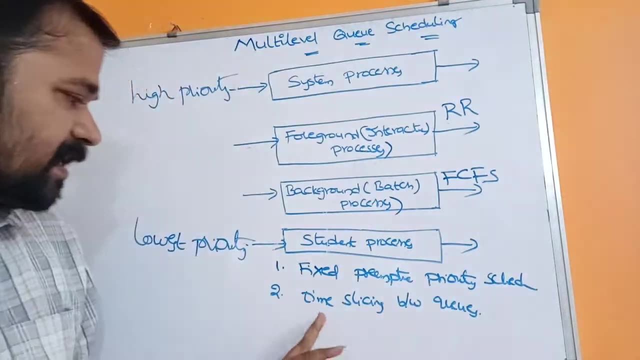 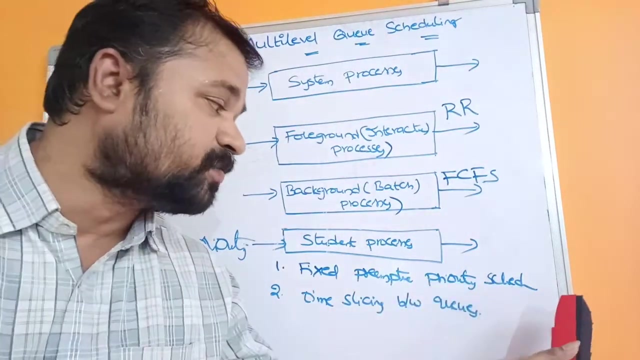 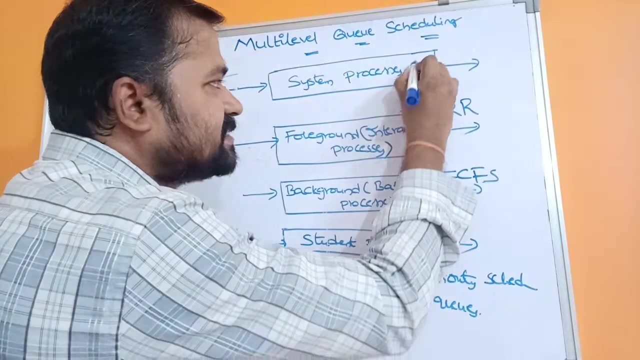 approaches. first one is fixed primitive priority scheduling algorithm, or we can also called as primitive priority scheduling algorithm, and the second one is by time slicing between the different queues. let's see the first one, fixed primitive priority scheduling algorithm. already some priorities are given to the ready queue. let there are five processes in this ready. 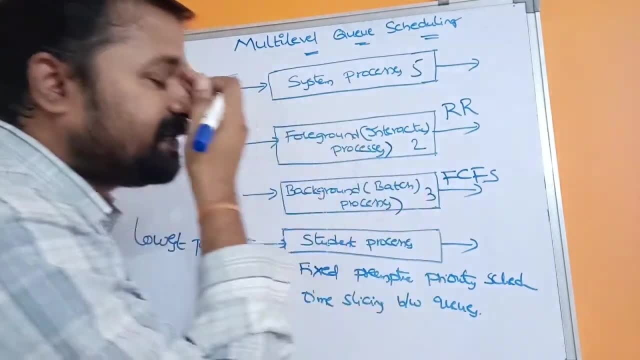 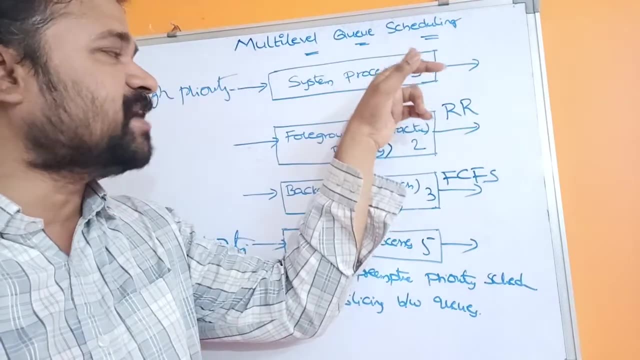 queue. let there are two processes in this ready queue. let there are three processes in the ready queue. let here we have five processes in the ready queue. so first we have to execute all the five processes in this ready queue. first we have to execute all the five processes in this ready queue. 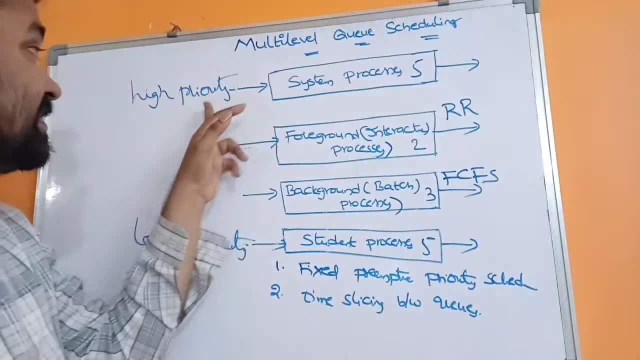 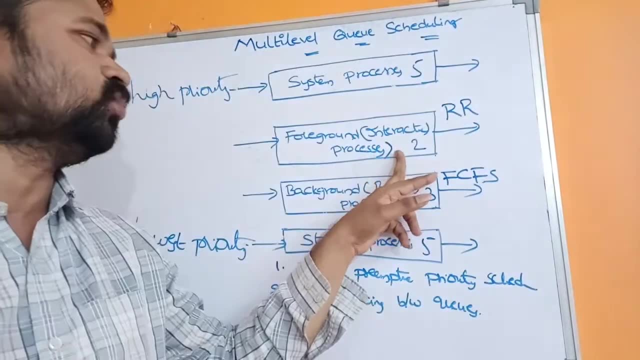 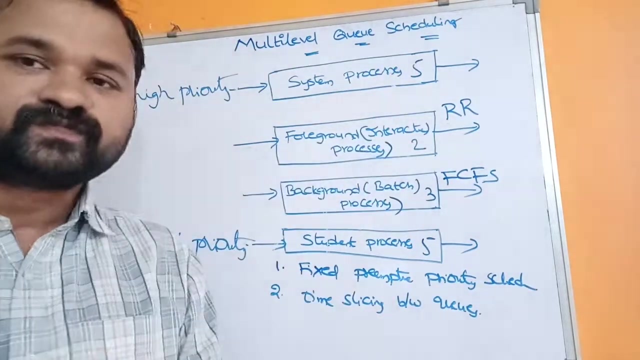 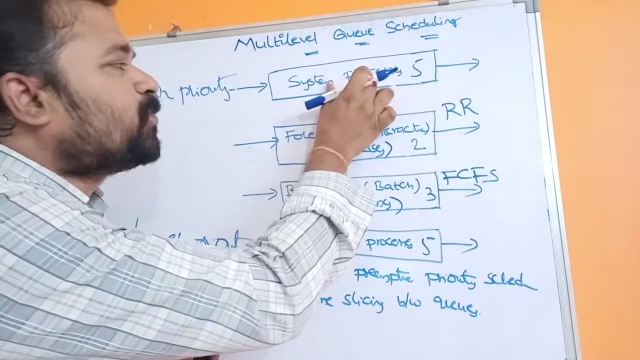 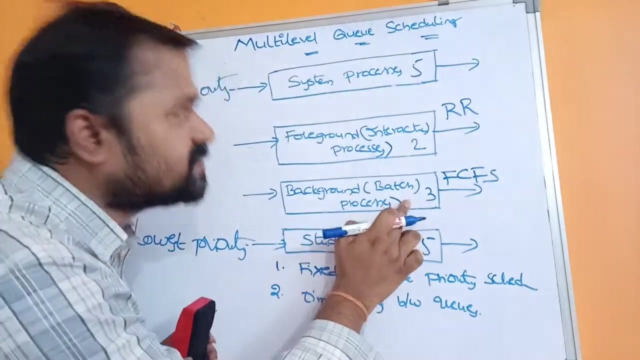 why? because this process is having highest priority. so once it is empty, then cpu control will be shifted to the next ready queue. now cpu execute the two interactive processes which resides in this ready queue. so here the point is: background process doesn't executes if there are some processes in this ready queue or in this ready queue so we can execute a background process. 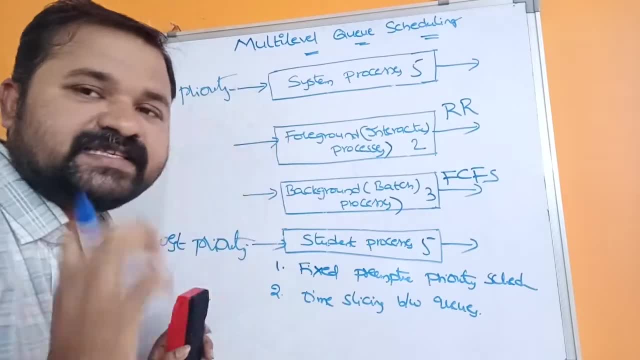 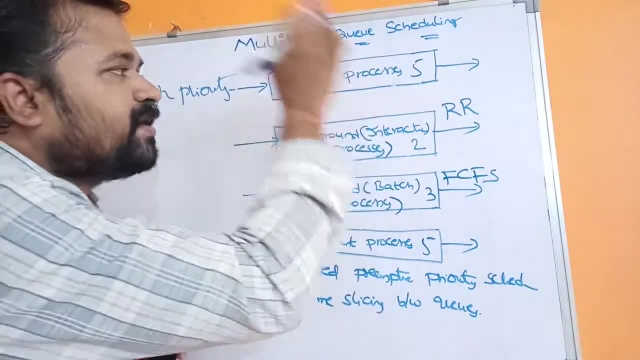 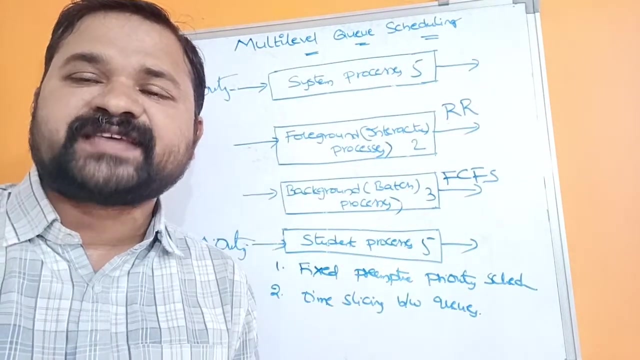 only when the first ready queue, as well as the second ready queue, is empty. so likewise we can execute a student process only when ready queue 1, ready queue 2, ready queue 3 is empty. so the major problem with this approach is starvation here. let us assume that more. 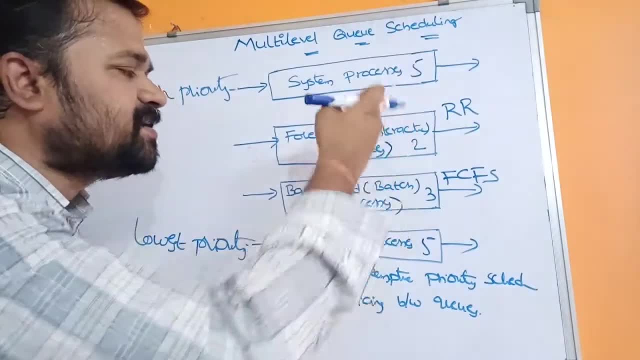 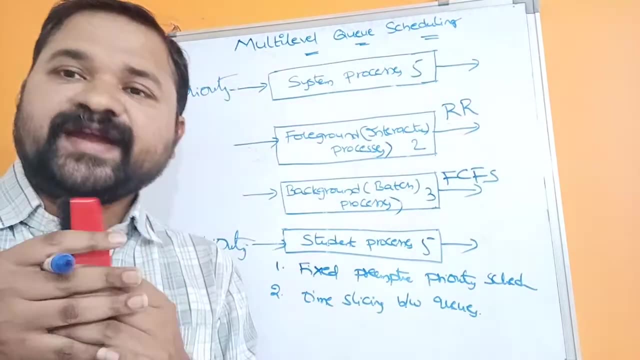 let us assume that more, let us assume that more number of processes are there in Radeq 1, Radeq 2 and Radeq 3, then student process will not get chance for its execution, So it has to wait for an infinite amount of time In order to overcome.